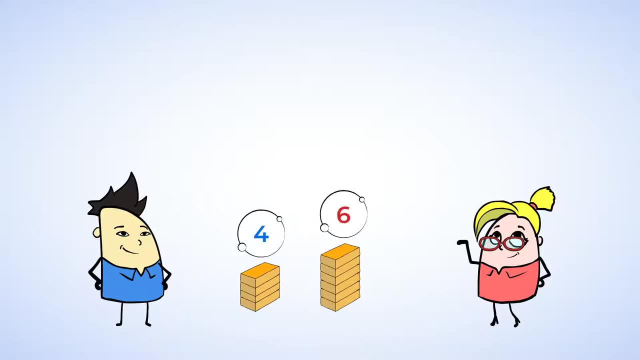 He has four blocks. Jenny's tower is taller than Chen's And look, Jenny and Chen both used all of their blocks And since Jenny's tower is taller, well, that must mean she has more blocks. This is because the word more 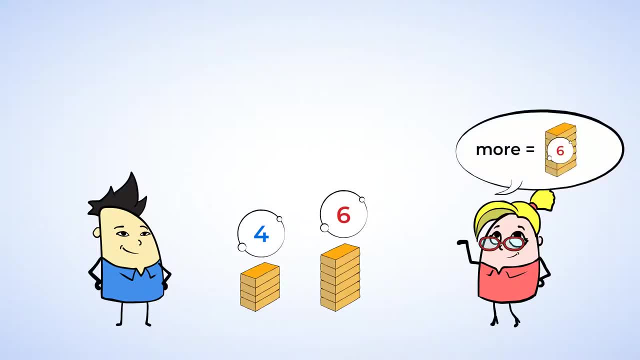 means a bigger number. Jenny had more blocks, so she had a bigger number of blocks than Chen. Well, six blocks is more than four blocks, so we can also say that six is greater than four. Greater than means bigger than. Ah and look, Eric and Latifa are also playing with blocks. 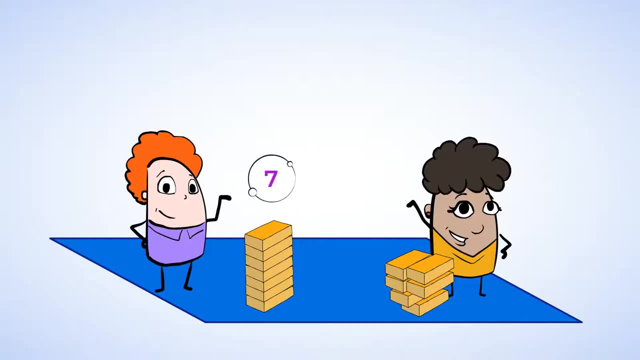 Looks like Eric has stacked seven blocks on top of each other and Latifa has stacked six. So who has fewer blocks in their stack? Fewer means less than or smaller than. So which stack is smaller? Well, Eric's stack of seven is taller and Latifa's stack of six is shorter. 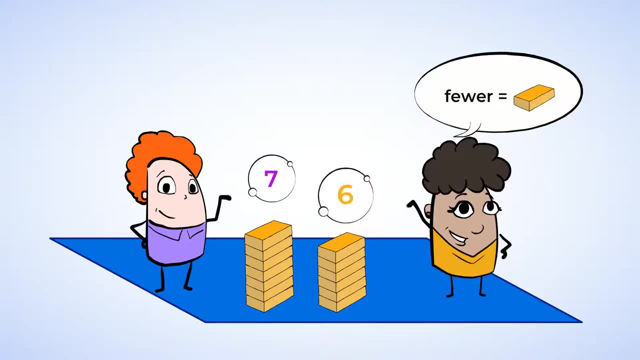 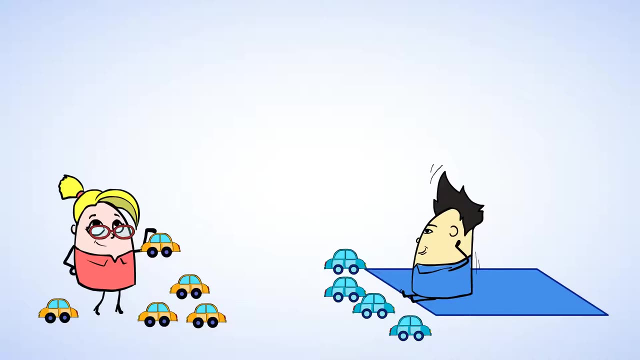 So Latifa has fewer blocks than Eric. Six blocks is fewer than seven blocks, So six is less than seven. Good job. It looks like Jenny and Chen are all done with their blocks. They're playing with cars now. Jenny is playing with five cars and Chen is playing with four cars. 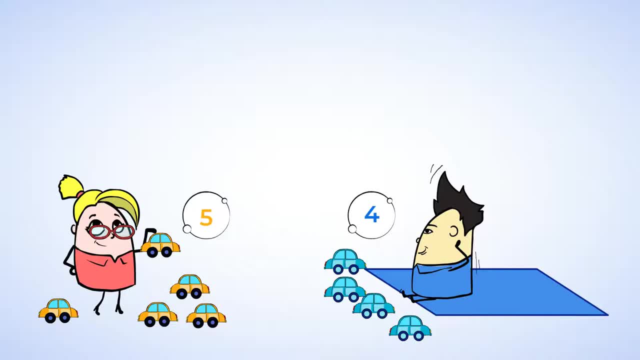 Is Jenny playing with more or fewer cars than Chen? Well, let's take a look. Wait a second. We can't build these cars up into towers. They would fall over. So what can we do? I have an idea. We can line up the cars to compare them instead. 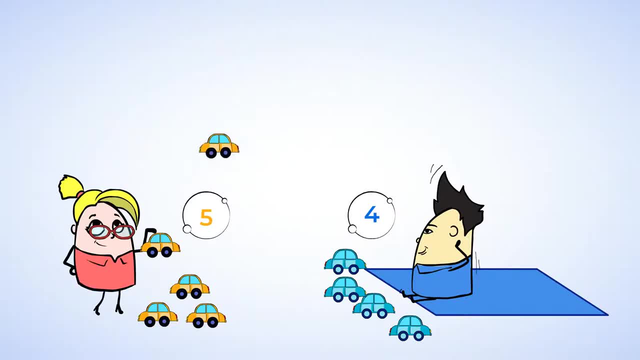 Make sure to line them up evenly. Now look, Here is one of Jenny's cars, and then here is one of Chen's cars. Okay, Another of Jenny's cars and another of Chen's cars. and we keep going And look. 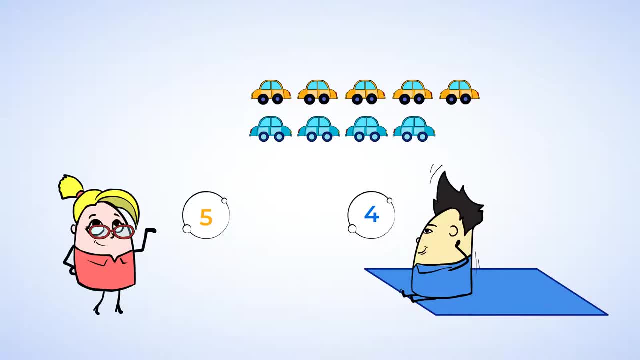 This is Jenny's last car, but Chen doesn't have any more. And now that we've lined up all the cars, don't forget why we did it. We wanted to know: does Jenny have more or fewer cars than Chen? Well, let's check together. 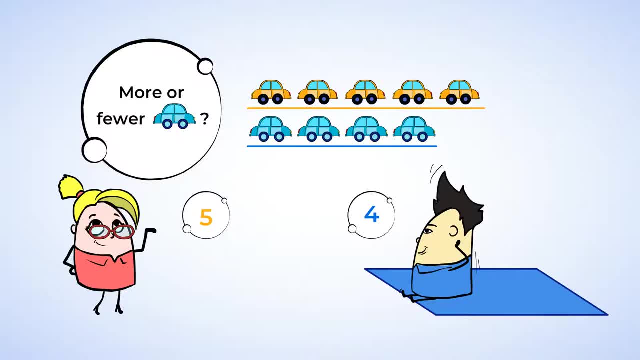 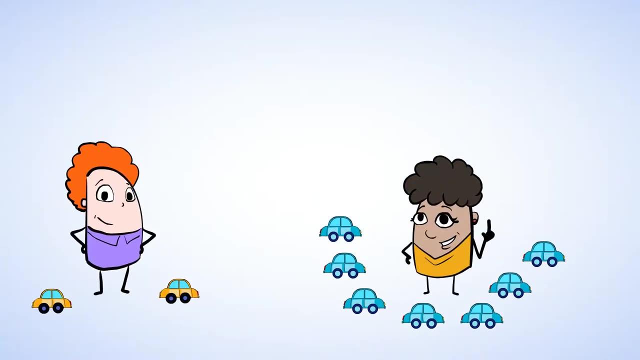 Is Jenny's line of cars longer or shorter? Jenny's line of cars is longer, So she has more cars than Chen. Jenny's five cars is greater than Chen's four cars. Look, Eric and Latifa joined the game. Eric is playing with two cars and Latifa is playing with seven. 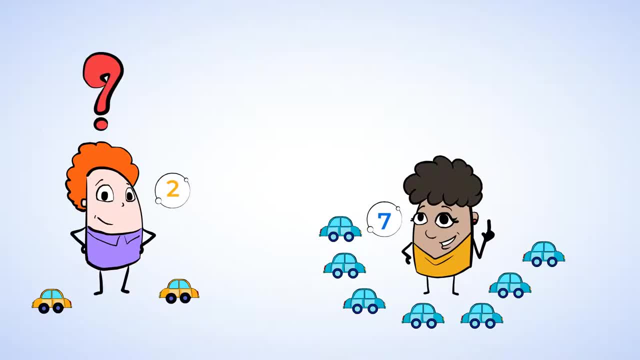 Is Eric playing with more or fewer cars than Latifa? Well, let's line them up. Line them up and find out. Well, here are Eric's two cars and here are Latifa's seven cars. Is Eric's line of cars shorter or longer? 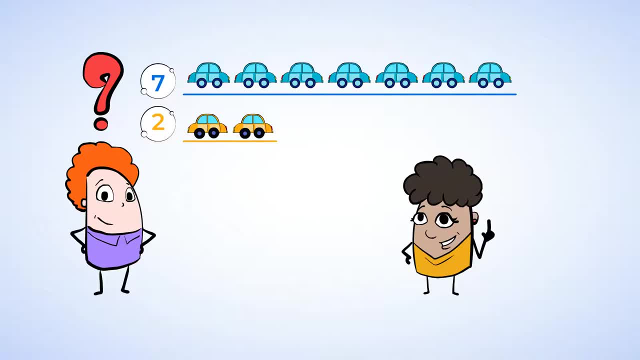 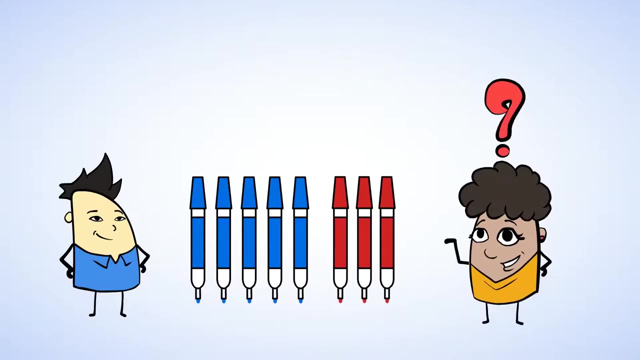 It's shorter, So Eric must have fewer cars than Latifa. Eric's two cars is less than Latifa's seven cars. Oh, Latifa and Chen moved on to drawing. now I wonder: Does Latifa have more markers or fewer markers? 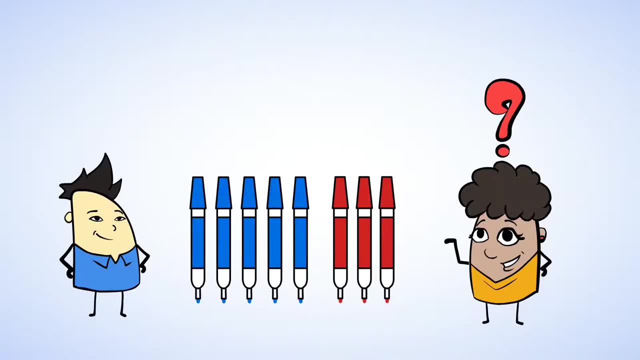 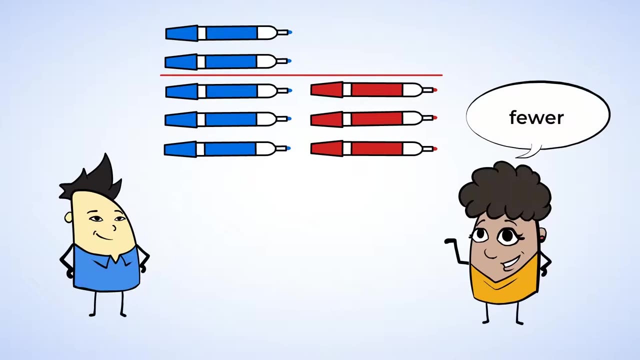 Well, just like with the blocks, we can line up the markers to see who has more. Let's look. Latifa's line of markers stops here, but Chen's keeps going. So Latifa has fewer markers than Chen. And how many markers does Latifa have? 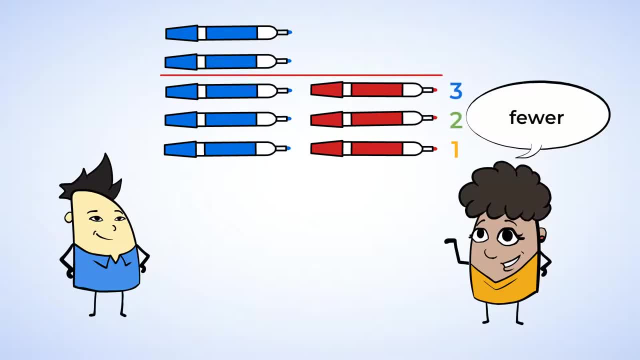 One, two, three. She has three markers. And how many markers does Chen have? One, Two, Three, Four, Five. He has five markers. Latifa's three markers is fewer markers than Chen's five markers. Three is less than five. 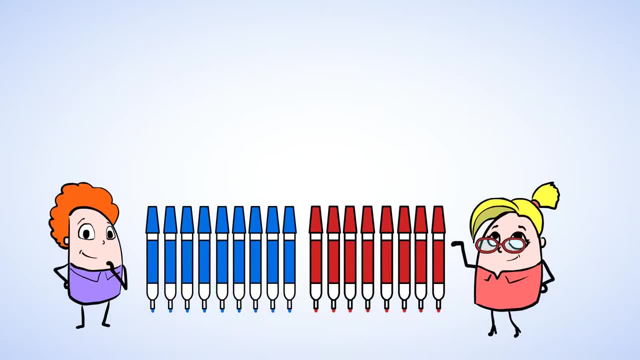 Ah cool, Eric and Jenny are drawing two. now Looks like Eric has nine markers and Jenny has eight markers. Does Eric have more or fewer markers than Jenny? Well, we could line up the markers again, But Eric and Jenny have a lot of markers and if we line them all up, well they might. 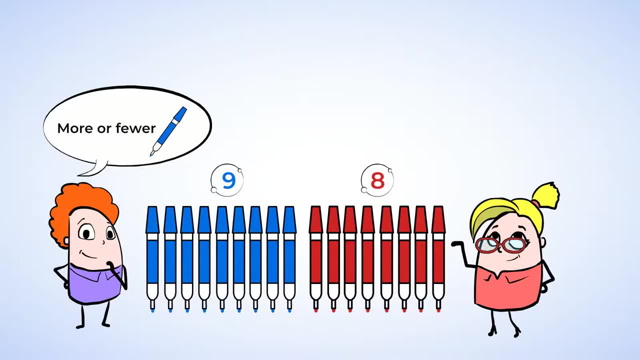 fall off the table. Hmm, I know We can use something to represent the markers. Look, We can use linking cubes. You can put these cubes together and take them apart to make different numbers. Let's make the number nine first One.